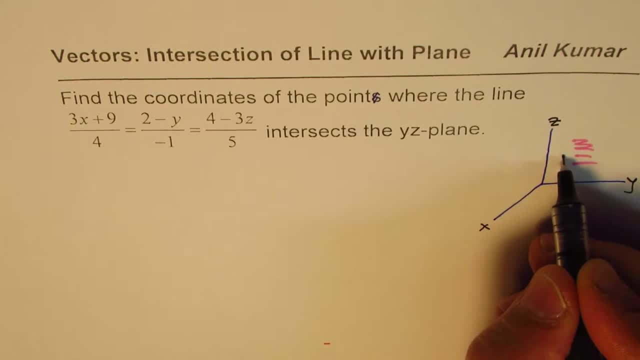 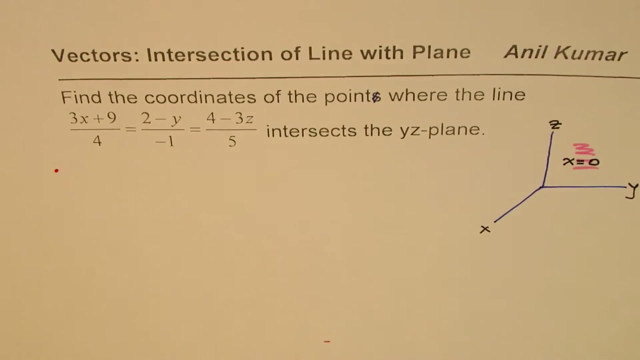 is on this plane. in that case the coordinate value of x should be equal to 0, right? So in this plane, coordinate value of x is 0. So that helps you to find the equation right. So that is the strategy. So we will do it in two steps. One is we will write parametric form. 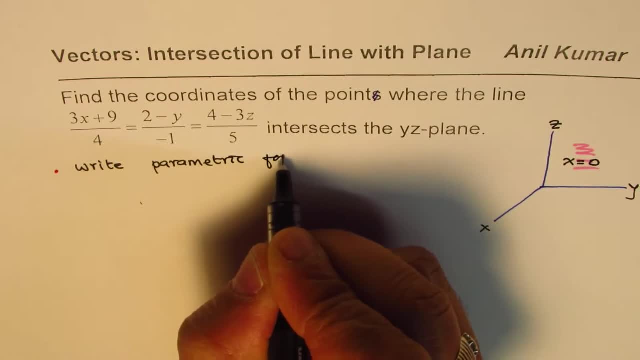 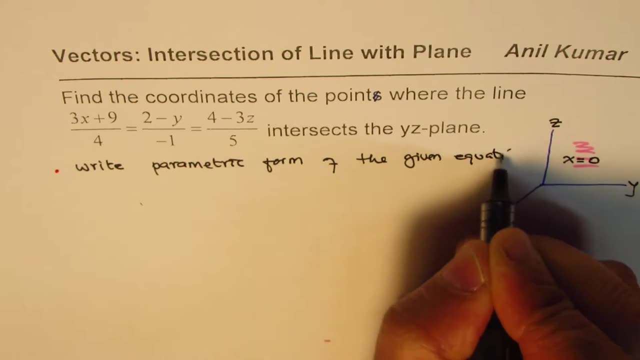 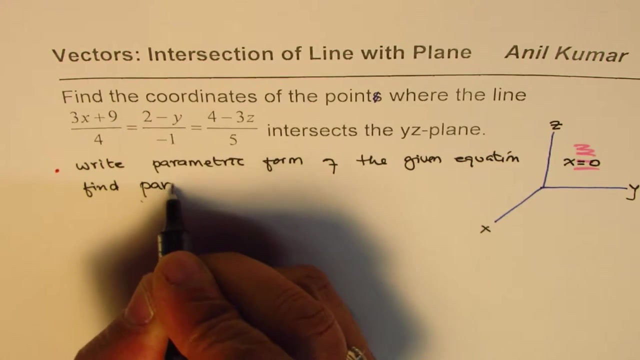 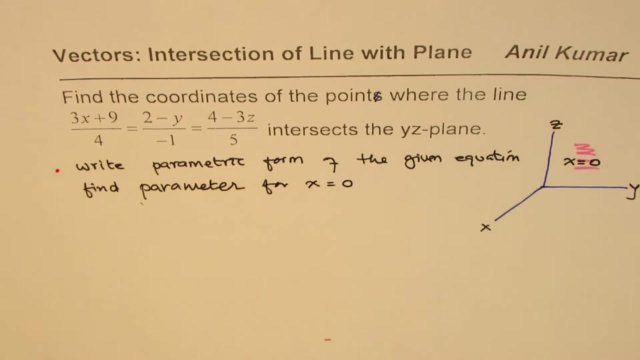 of the given equation. and second, we will find or calculate parameter for x equals to 0, right. So these are the steps involved. So I hope now, with these steps, you should be in a position to solve the question. You can pause the video answer and then look. 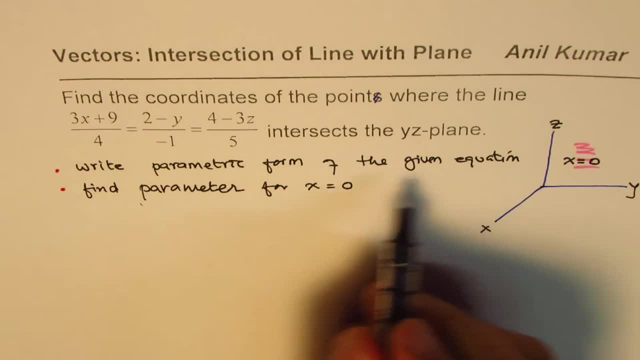 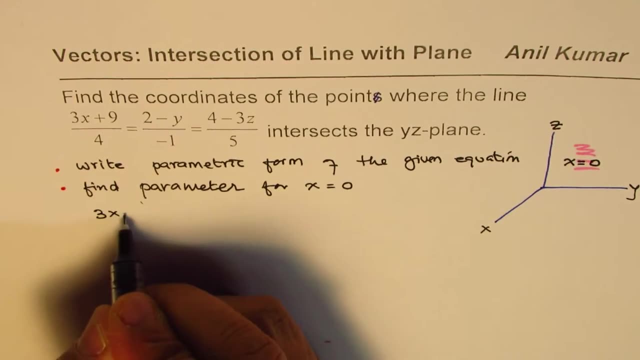 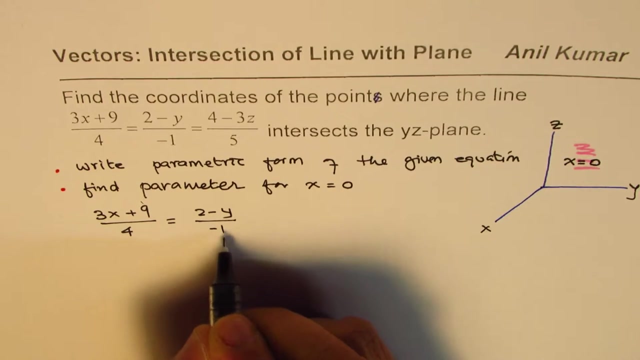 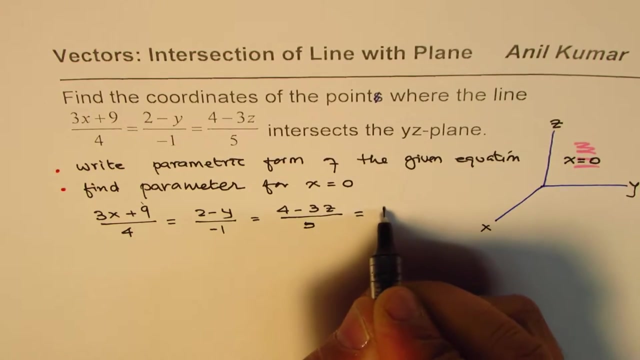 into my suggestion. Well, how to write this in parametric form? So these are the. let me copy this equation first. We have: 3x plus 9 over 4 equals to 2 minus y over minus 1 equals to 4 minus 3z over 5.. Let this be equal to parameter t, right? So that is. 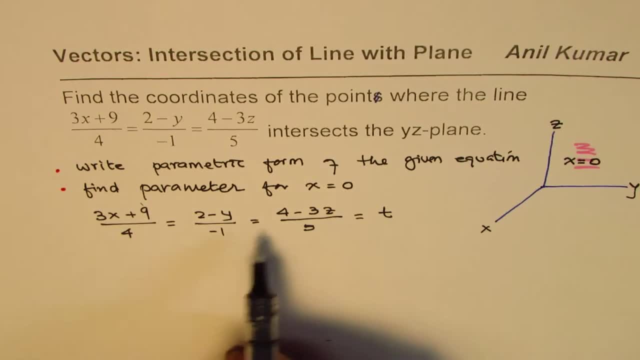 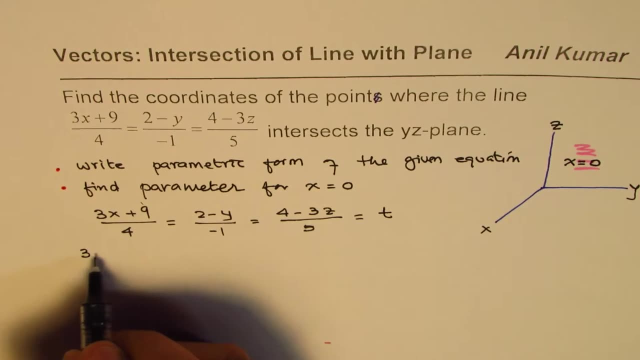 the key. So once you write this as parameter t, right, then you can convert easily into parametric form. So let's look into the first equation. We have first equation as 3x plus 9 over 4 equals to 3x plus 9 equals to 4t. or we can isolate x, So we can say 3x equals to 4t minus 9, and then 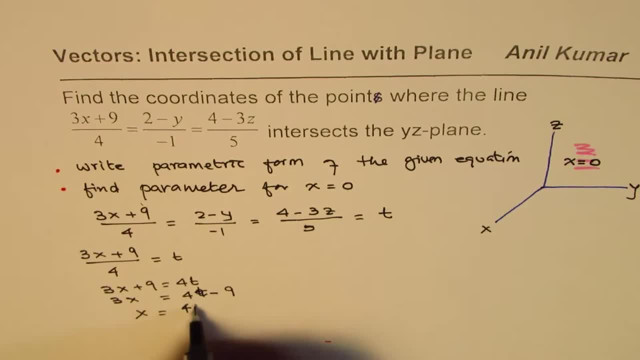 divide by 3.. So x equals to 4,. I mean this is t 4t minus 9 divided by 3.. So that is how we can get parametric form. So x is equals to this. Similarly we can write others also, right? So? 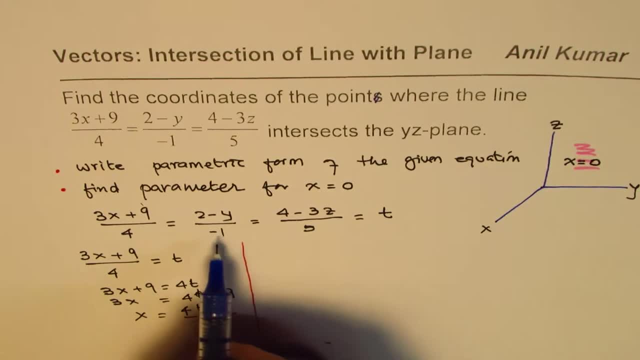 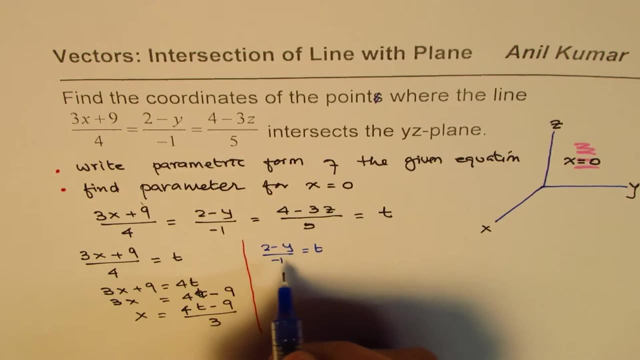 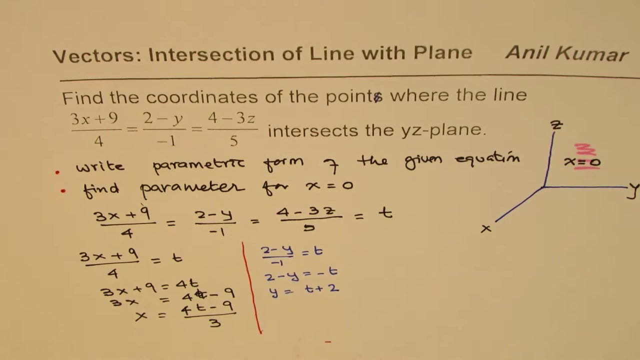 I'll not show these calculations now, but in fact give you what y should be. or let's do it okay: 2 minus y over minus 1 equals to t, and that gives you 2 minus y equals to minus t. Bringing y to this side, we get and t to this side, we get t plus 2.. So that's the second equation And the third one. 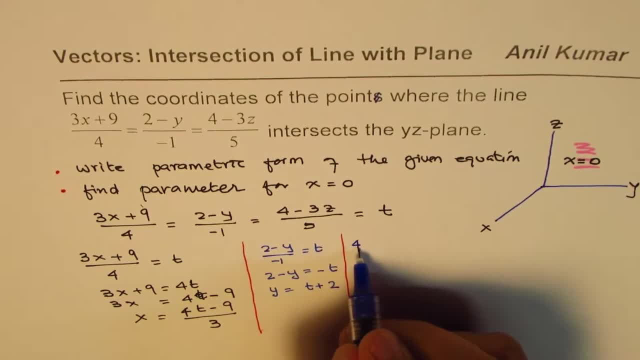 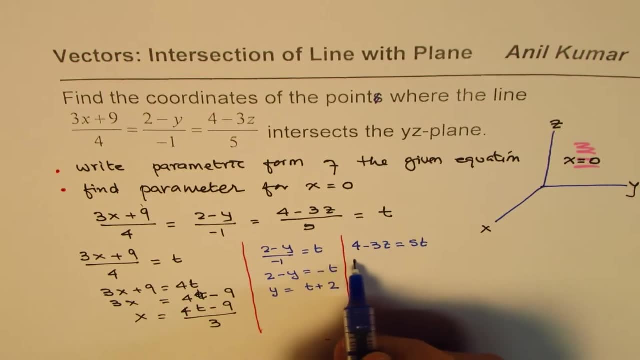 we'll do. we'll cross multiply So we have 4 minus 3z equals to 5t, and bringing z to this side, So we get 3z equals to and 5t to this side, 4 minus 5t or z equals to 4 minus 5t over 3 right, So that. 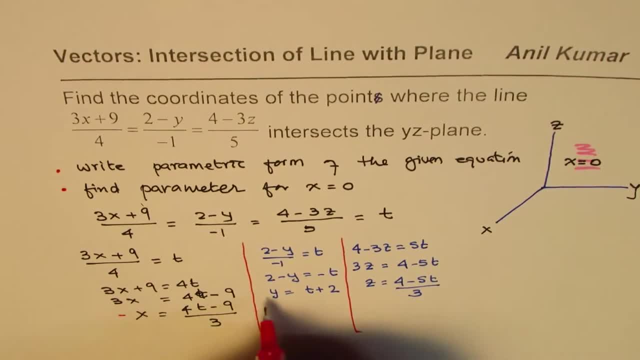 becomes the parametric form. So this is for x, this is for y and that is for z. Now what do we need? We need to make x zero, right? So if x is zero, what is t? That's the whole idea, right? So let's get back to, and then we'll calculate y and z, right? So the idea here is to: 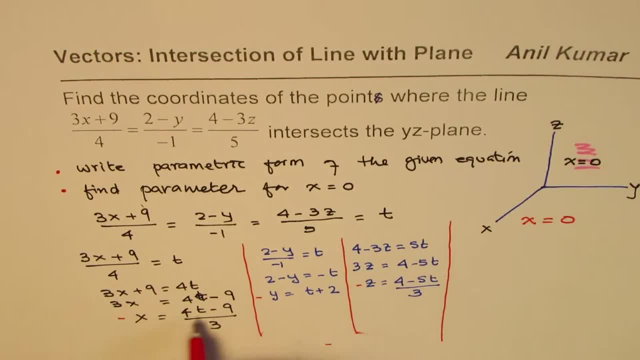 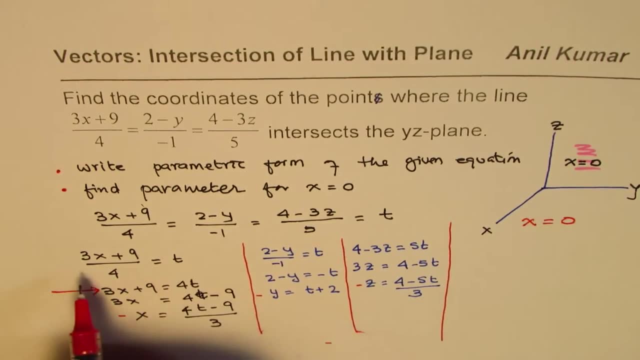 make x equals to zero, We could have used this equation also. This is better to use actually. So the equation is, or even this one, So the equation is. so what we will do is: actually: you might do a calculation mistake here, So that is very safe to use. So in this equation, which is: 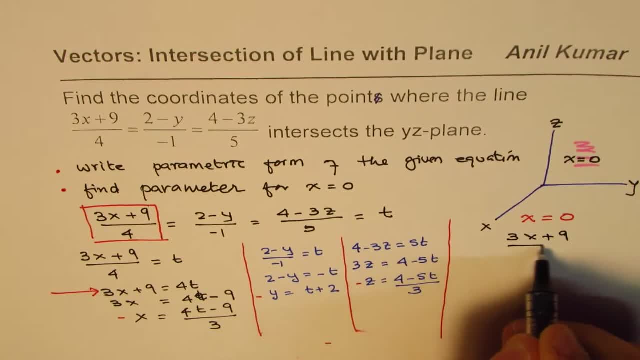 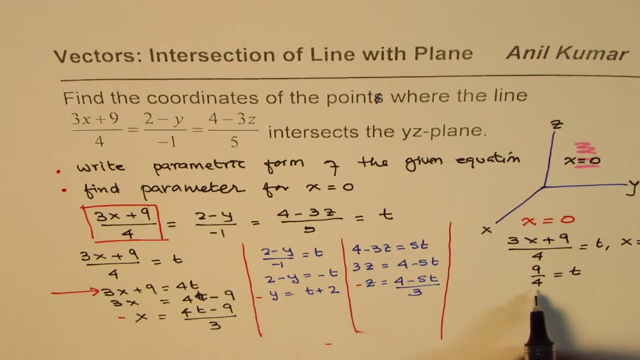 for us, 3x plus 9 over 4 equals to t. I'm going to substitute x equals to 0, right. So if I write x equals to 0, I get 9 over 4 equals to t, right. So the value of t is 9 over 4.. Now what do you need? 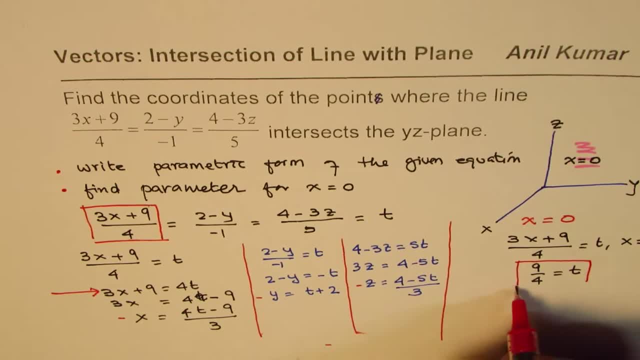 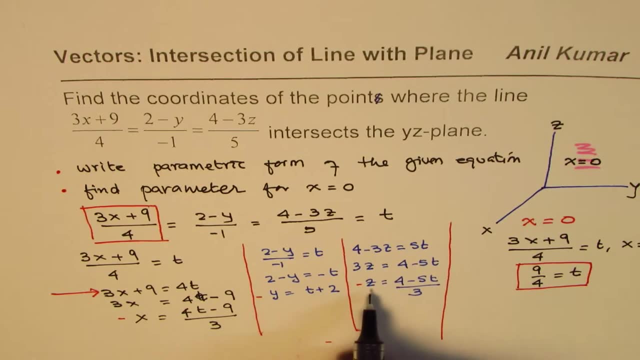 to do. You need to substitute x equals to 0 over 4, right? So there's this. kind of fractions may be difficult at times to work with, Anyway. so substitute t equals to 9 over 4 and get y and z. okay. So that's the whole idea. So what we get here is, from here, y equals to 9 over 4 plus 2. 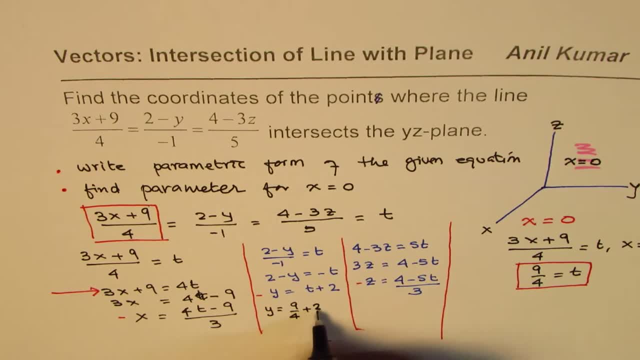 right, Which you could write as: 4 times 2 is 8.. 8 plus 9 is 17.. So you get 17 over 4 as your value. As far as z is concerned, z will be equals to. let's rewrite: 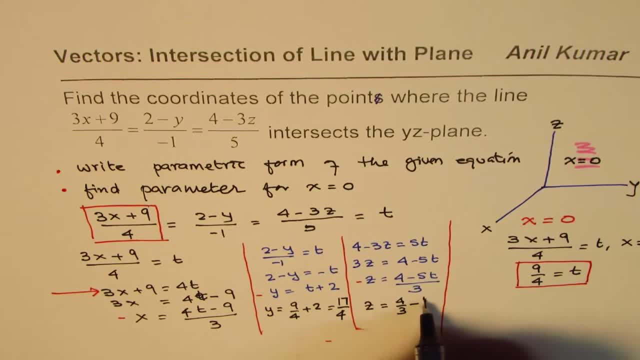 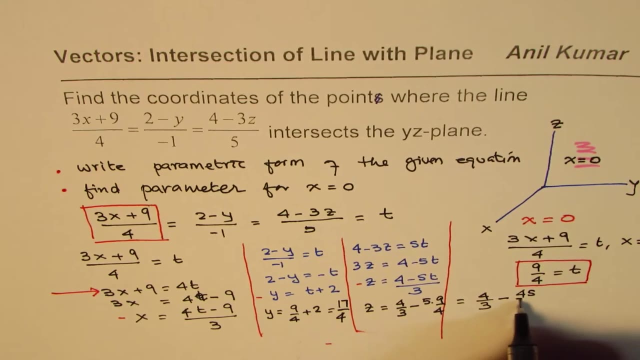 this as 4 over 3 minus 5 times 9 over 4. okay, This is kind of tricky. okay, Let's extend this side: 4 over 3 minus 9 times 5 is 45 over 4.. So with common, 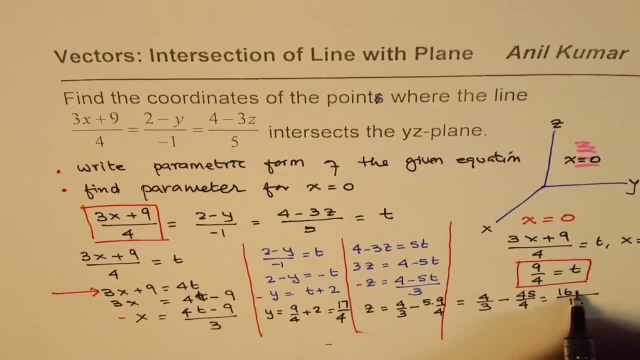 denominator of 12, we have 16 minus 3 times 45. So it is 15, 5 and 1, 12, 135, right? So now we'll take away 16 minus 135. So we get negative. This number is bigger. So 15 take away 6 is 9 and 2. 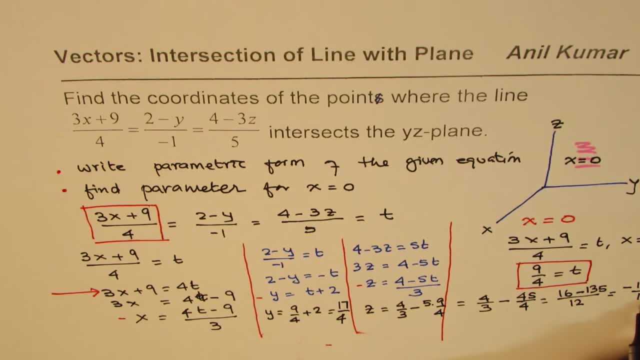 take away: 1 is 1.. So we get 1 1 9 over 12, correct, And that gives us the coordinate point. So our answer here is: let me shift this page a bit on the right side, So we have x value as 0. 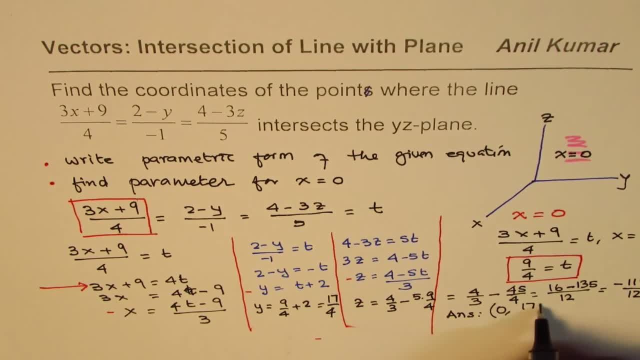 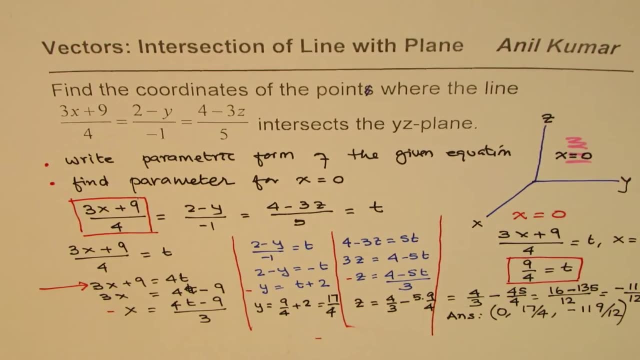 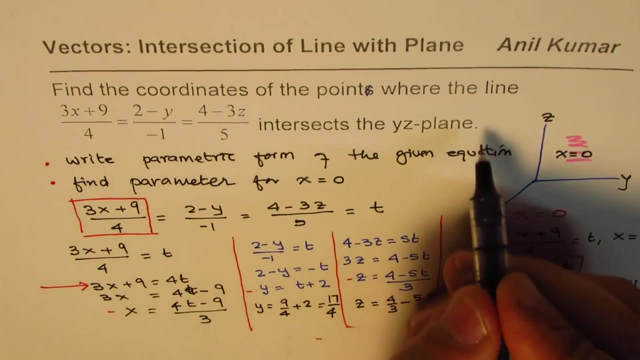 right, Y value is 17 over 4 and z is minus 1: 1, 9 over 12 right. So that is how you can find the solution to this. Now, as an added exercise, what you can always do is find the points where it. 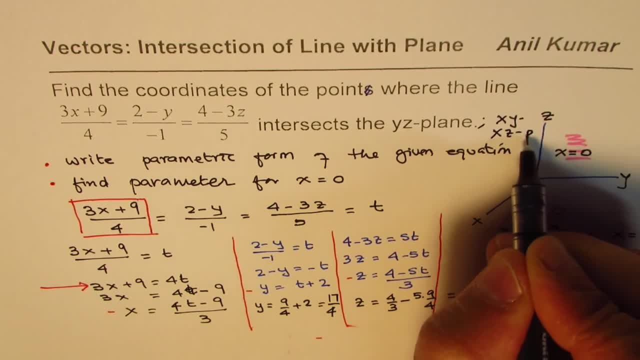 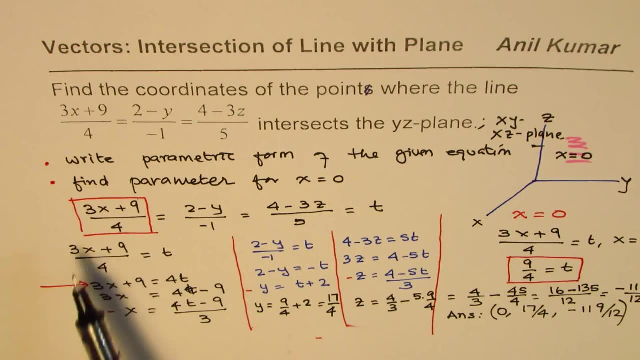 is less than or equal to 0 and x, z, plane right, So that you could do as a practice question for the same. So, as you have seen here, we need not really simplify this one. So we need to write complete parametric form to save time. It works. So that's kind of a learning from this, from this. 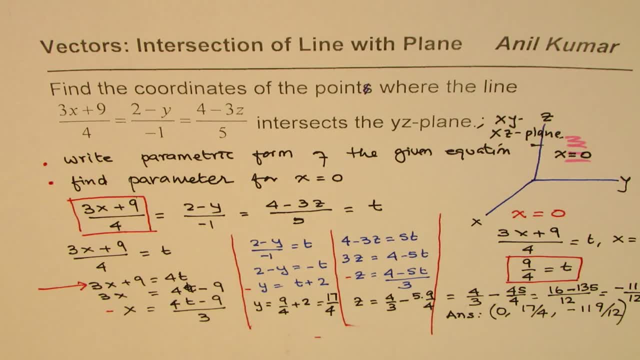 video. I hope that helps. Thank you and all the best.